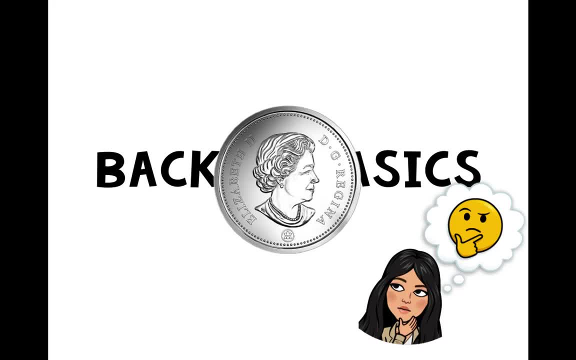 Okay, one die, Alright. so let's take it back to last year. What do you guys remember about finding probability? Okay, so I know when people say, when you flip a coin, what is the probability? And a lot of you guys say it's a 50-50 chance, right? 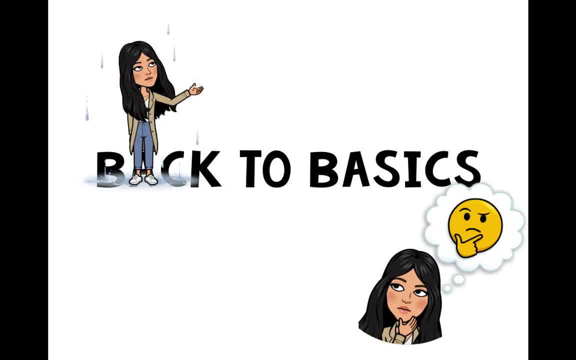 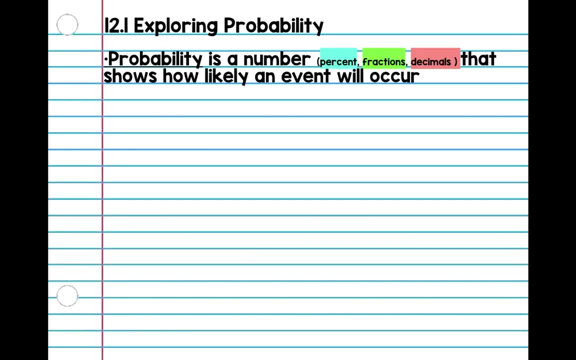 Because there's two sides, Or sometimes on the weather they go. there's a 15% chance of rain today, So that is all probability, Okay, so let's begin. So what is probability? Probability is just a number: percent, fraction or decimal. 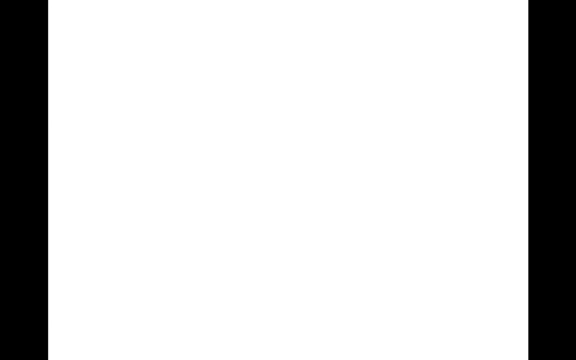 that shows how likely an event will occur. Okay, so let's look at how likely. So here we have zero and we have one. These are the numbers we're going to be working with for this entire, And if it's half of it, it's one half. 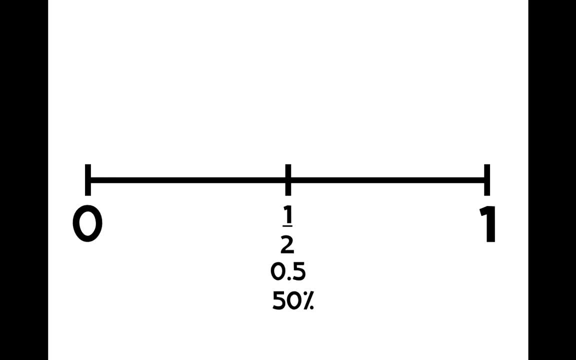 Okay, so in decimal form we have 0.5.. And then in fraction form, you know it's 50%, And then, as for one, we have one and 100%, And then zero is obviously zero. So anytime something is certain, it's 100%. 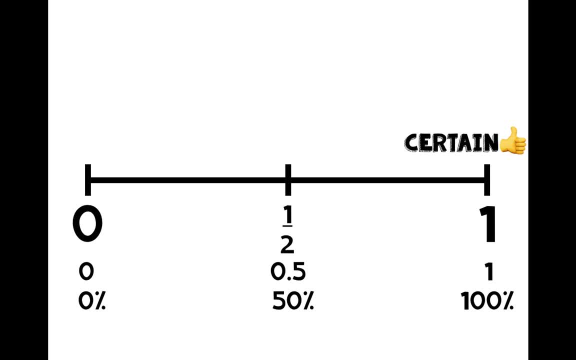 So, for example, tomorrow there's 100% chance that we have school Because it's Monday, right? Any For 0%, impossible means it can't happen. For example, there is a 0% chance that you guys are going to PCC today. 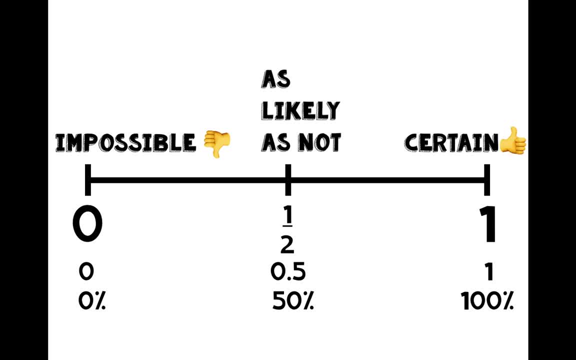 because you're not allowed to So anything in the middle. we call it as likely as not, And we use the word likely when we're talking about probability. So from 50% to 100, we say likely, And then from zero to 50%, we say it is unlikely. 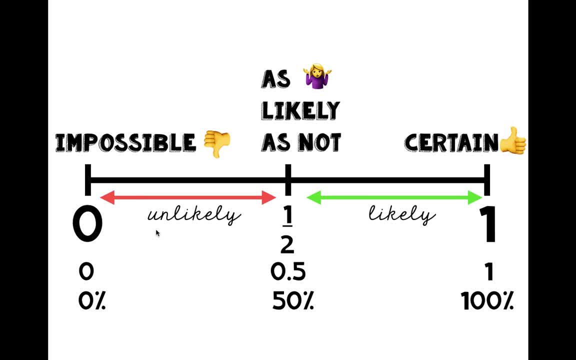 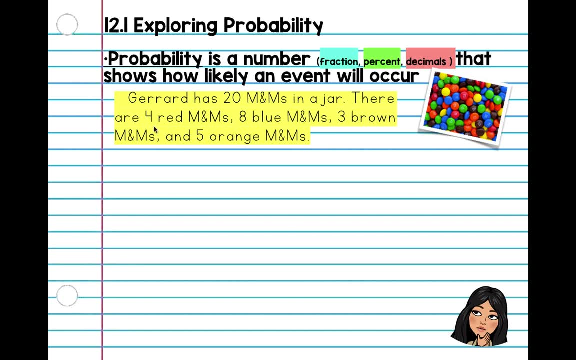 Okay, And that's just pretty much the basis of what you have to know with using likely and unlikely. Okay, so let's have, like, some scenarios going on. Gerard has 20 M&Ms in a jar and there's four reds, eight blues, three browns and five oranges. 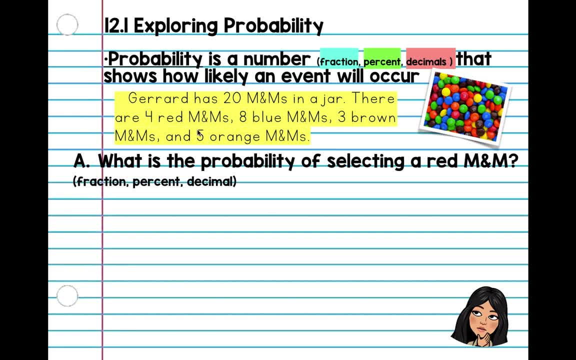 Question number one says what is the probability of selecting a red M&M. So red is right here. So let's start with our fraction form Before we even begin. there's a formula when calculating probability: P of n equals number of favorable outcomes over total. 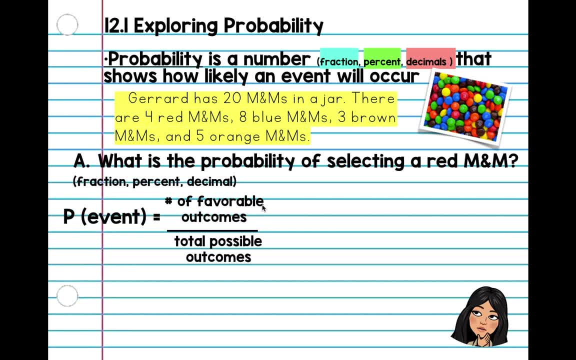 possible outcomes. So this is really easy. It looks confusing, but it's not So. the reason why we use P is for probability, So let's start with our event. What is our event? It's basically what they're asking. So the probability of getting red equals. 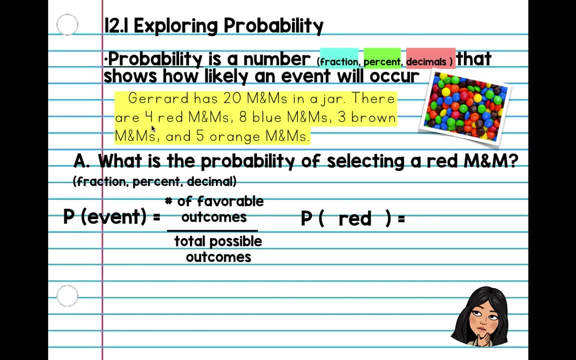 and you just have to look What is the favorable outcome. We know it's four, So four over, and our total possible outcomes is 20.. And there you go, guys. But we know we can never leave it as a fraction. that's not simplified. 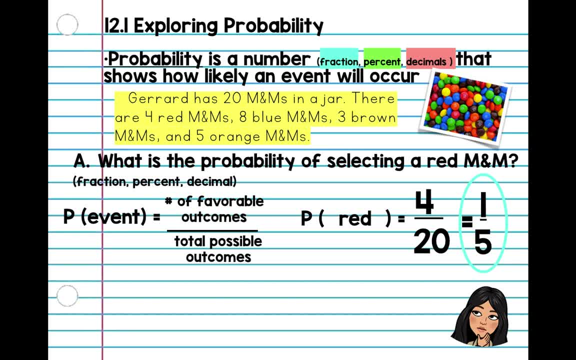 So our answer is one-fifth. Okay. So now that we have fraction, let's do percent and decimal. So we know, when we did ratio back, like last year, we used something called a scale factor And we tried to figure out how to get from five to 100,. 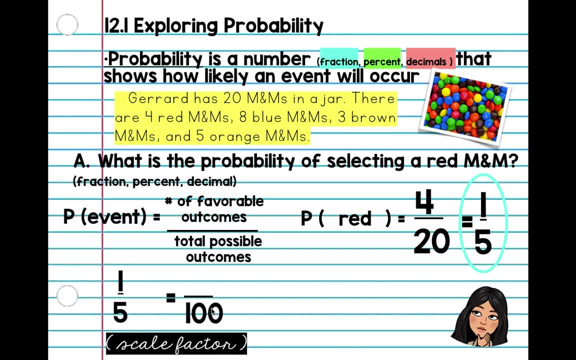 or figure out. what do we multiply to make the fractions equal? So our scale factor here is 20, right, Five times 20.. So what we do on the bottom, we do on the top. So our fraction equals 20.. 20 over 100, meaning our percent is 20%. 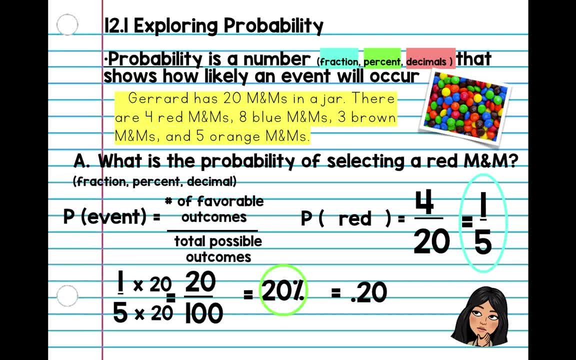 Once we have our percent, we can find our decimal, which is 0.2 or 0.20.. Two-tenths or two, 20 hundredths, Okay, And that is all you have to do, guys, to find probability. 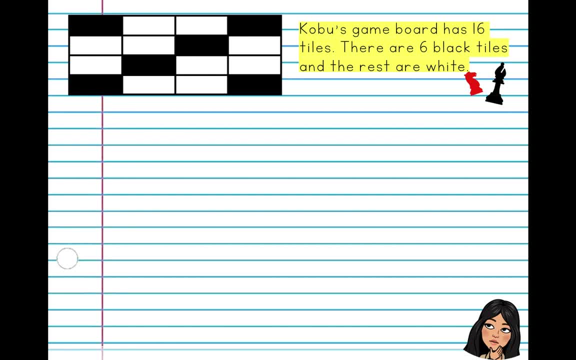 So let's have another situation. Kobu's game board has 16 tiles. There are six black tiles and the rest are white. So what is the probability of selecting a white tile? Okay, So here we have. probability of getting white is let's look how many we have at white. 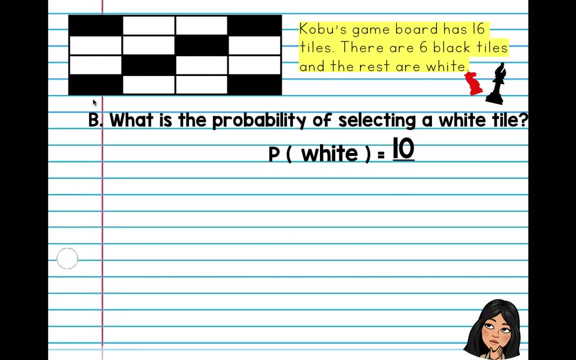 We have 10. And our denominator is our total outcome, which is 16.. So let's just reduce our fraction by two. Our fraction is five-eighths. Okay, Easy stuff. Now let's move on to our percent and our decimal. 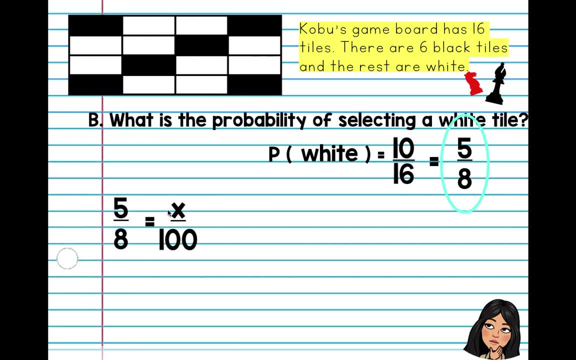 So five-eighths equals what over 100?? So when we did ratio we had to cross, multiply and do this whole formula. but we don't have to do that, We can just solve it normally. So in order to find how or what number is over 100, the percent. 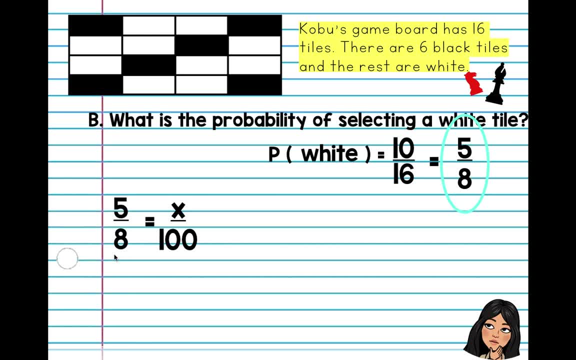 you just have to divide five, the numerator, by the denominator. So we take five, divide it by eight, and there you go. So we know eight can't go into five. so that's where decimals come in. So eight can go into 50, six times, which is 48.. 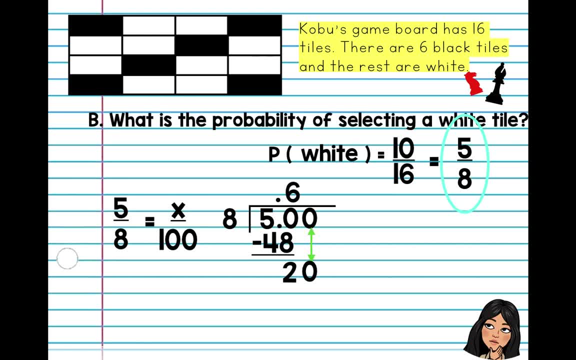 50 minus 40 is two. Bring down our zero Eight can go into 20 twice, which is 16.. Okay, Let's go one more time. and the reason why we want three is that we can determine if we need to round up or not. 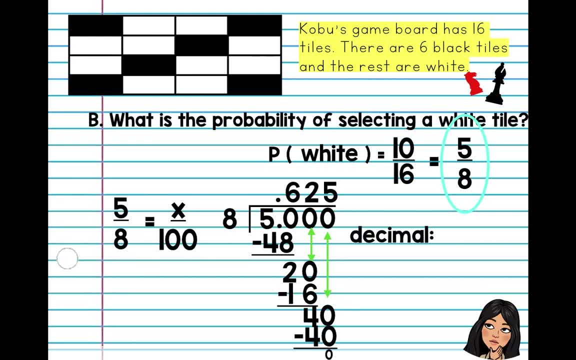 So eight can go into 45 times. We have no denominator, So now our decimal is .625, but we really just want to keep it at two numbers. So we know we just have to round this number up, because this number is five. 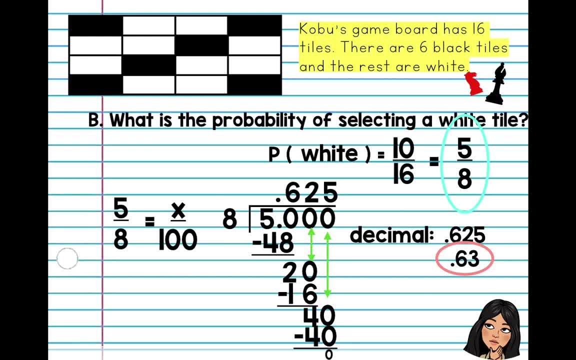 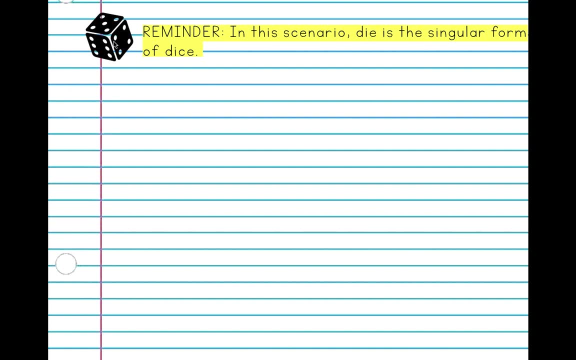 So our decimal is .63.. There you go. So once we have our decimal, we can just quickly find our percentage, which is 63%. Okay, Is everyone following along? All right, So let's do one more situation. So in this scenario, we are using a die which is just one dice. 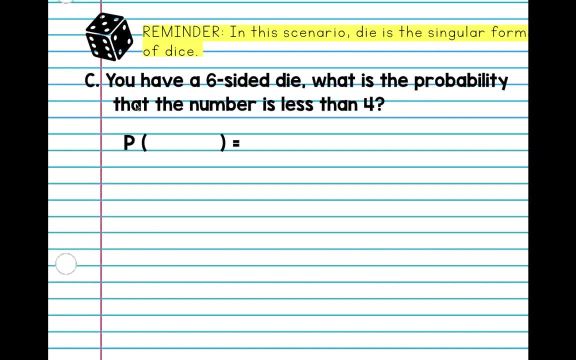 Okay, You have a six-sided die. What is the probability of that number being less than four? So our answer of probability or event is a number less than four. In this case, you can write: n is less than four, So let's count. 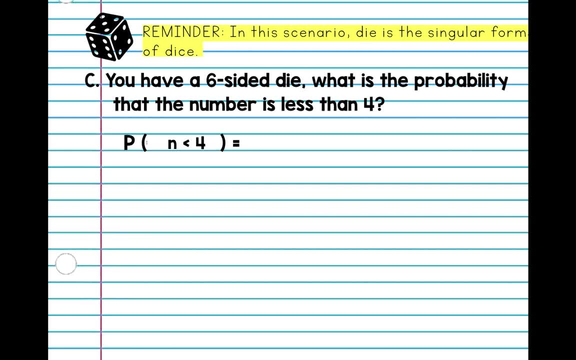 Okay, So we're going to do all the numbers less than four on the dice. We have one, two and three. Four doesn't count because that's equal to four, So we have three. So we have three numbers over our total, which is one, two, three, four, five, six. 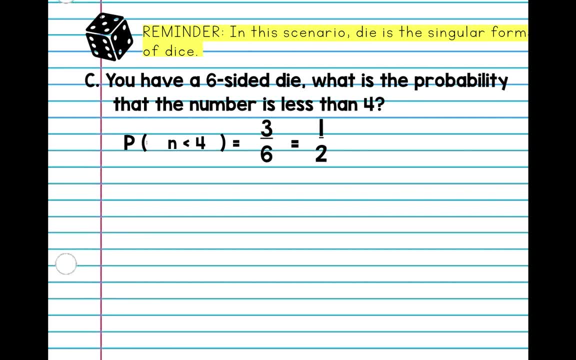 So our fraction is one half, And that's easy. One half is easy, We know it's 50% And our decimal is .5 or .50.. Okay, Let's do one more. What is the probability that the number is showing six? 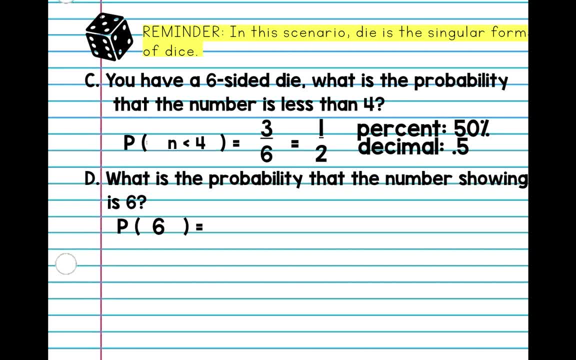 Okay. So obviously we know that there's only one number, that's six. So it's one sixth, Okay. So now let's go back to what we just did on the last slide. We just multiplied one by six, Okay, So we know that we have to put .0 there. 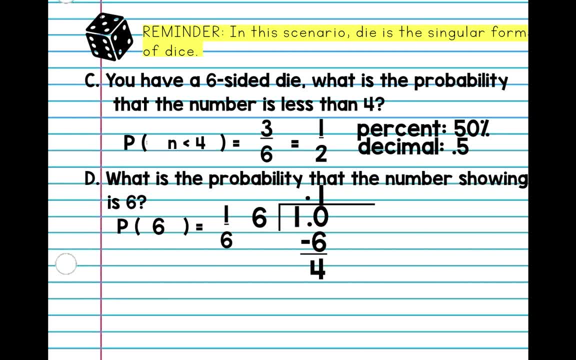 Six can go into ten one time. So bring down the zero, So six can go into 46 times, which is 36.. Okay, So we have a pattern, So we know it's going to be 1.6666 all the way.